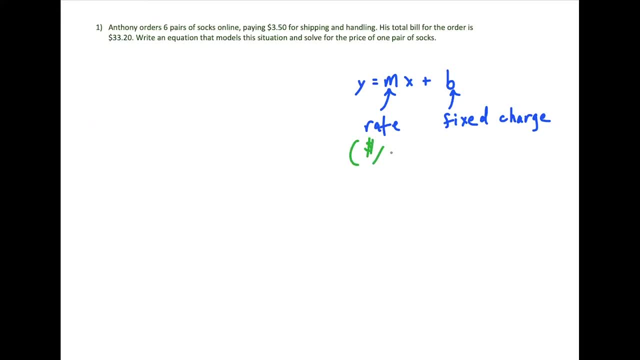 in dollars for one pair of socks. So the dollars per pair of socks And the fixed charge here represents the cost of shipping. And now to think about what x and y represents: x represents the cost of shipping And y represents the cost of shipping. 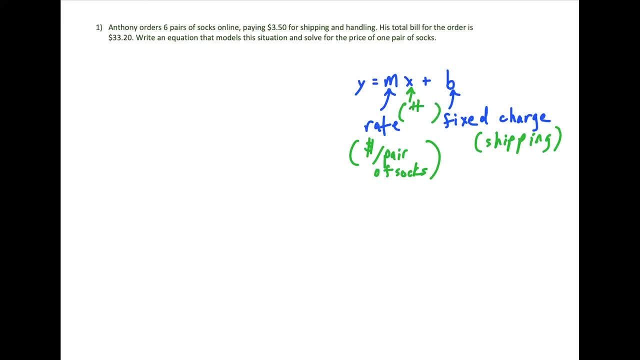 number of socks that we're buying. so the number of socks, and that's the old school symbol for number. so number of socks, and then this represents the total cost. so y is the total cost. so then all we have to do is just extract all the information from the word problem here and 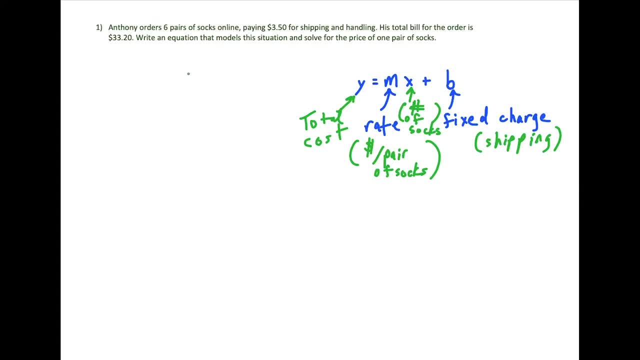 set up our equation. so we know that anthony orders six pairs of socks. so after the equal sign- and let's go ahead and change colors here- so after the equal sign, we have m times six. the three dollars and fifty cents that he's paying for shipping and handling represents b, the fixed. 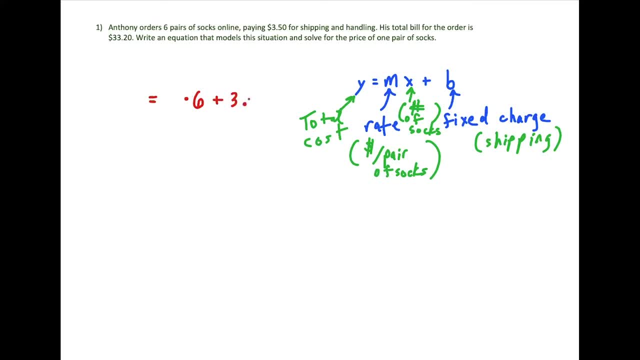 charge. so we have plus three dollars and fifty cents, which we'll leave out the units for dollars, we'll just write 3.50, but just you can imagine the dollar sign and then the total bill for the order is three dollars and fifty cents and then the total bill for the order is three dollars and fifty cents. 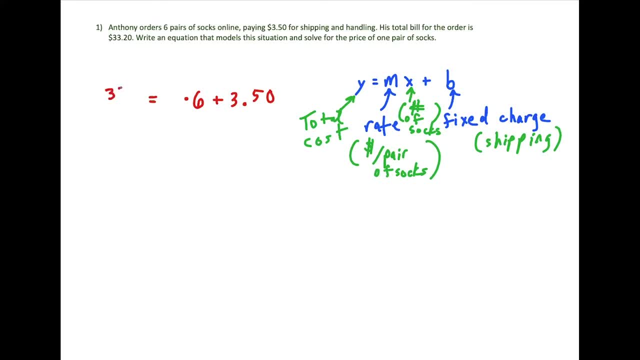 33.20. that represents the total cost. and the question is: well, we have to first write an equation, which is what we're doing, but we want to solve for the price of one pair of socks, so that's the rate that we're solving for. so we have m. 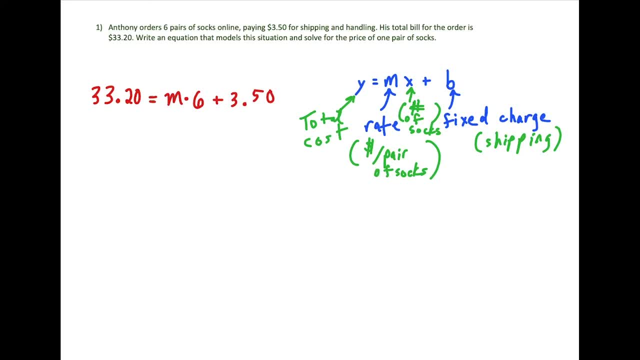 times six. so we want to know how much is it for just one pair of socks? so if we clean up this equation a little bit, we have 33.20 equals 6m plus 3.50. so all we have to do is just solve this linear equation for m. 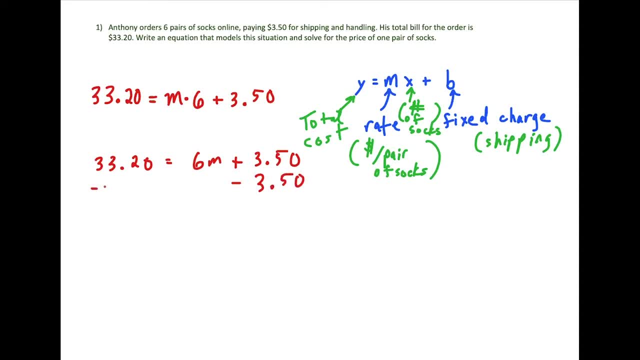 and we'll be done. so we're going to subtract 3.50 on both sides and just a little commentary here. for these questions, the hardest thing is setting up the equation. solving the equation is not so bad, but you just have to know where the variables go when. 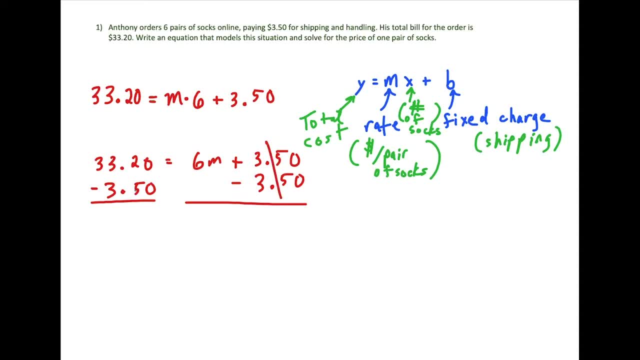 you're setting these up, so these two cancel and we could use a calculator. but this isn't so bad. we want to practice our old school math, so we could change 33.50 to a 32. that makes this a 12. so then we have 12 minus 5 is 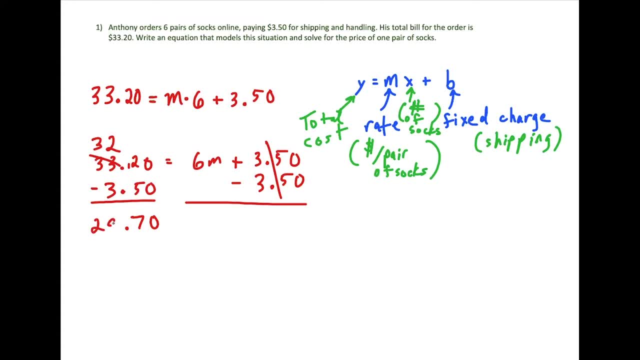 7 and now 32 minus 3 is 29, so we have 29.70 equals 6m and divide both sides by 6 so we could use a calculator. but this isn't so bad we have. 6 goes into 29 four times. 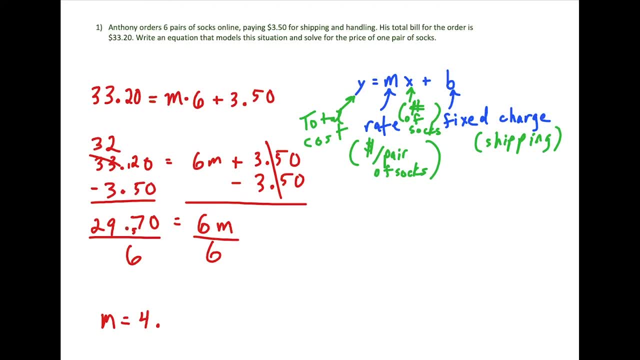 and there's a remainder of five. so we just throw our decimal in: six goes into 57 nine times, with a remainder of three, because 54 is as close as we get and 54 is three units away from 57. and then 6 goes into 35 times. 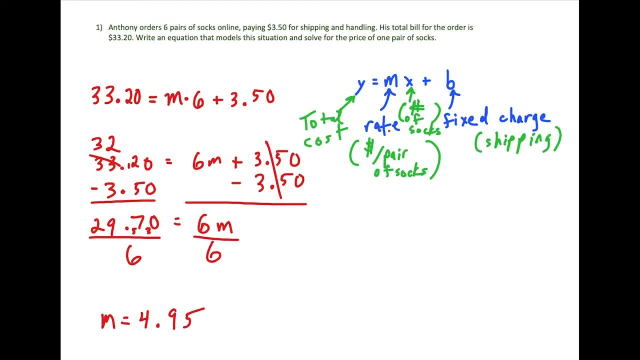 so now we just have to interpret this. m represents the rate, which is the dollar amount for one pair of socks. so this tells us that the price of one pair of socks is 4.95. so we're going to have to calculate the rate of the price of one pair of socks. 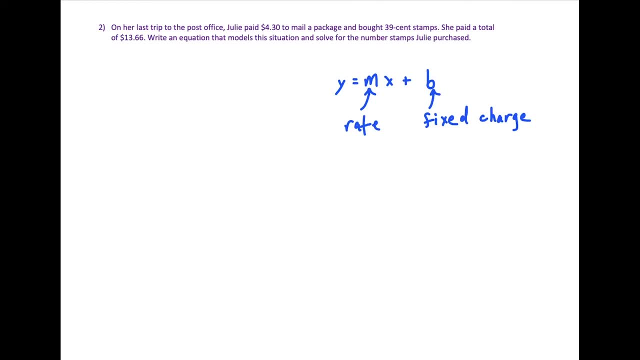 okay for question two, it's the same idea but take a second to read through this. but now we have julie at the post office and she paid 4.30 to mail a package and bought 39 cents stamps and we have the total for her bill and we want to write an equation that models this. 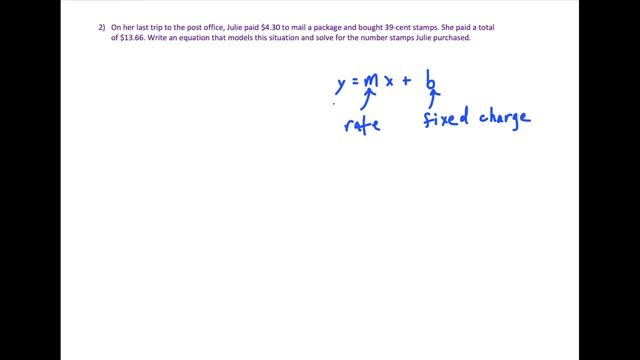 situation and we want to solve for the number of stamps that julie purchased. so if we just kind of fill in this information here, the rate represents the cost for one of the stamps. so in this case here the rate represents the dollar amount for one stamp. okay b, the fixed charge represents how much she paid to. 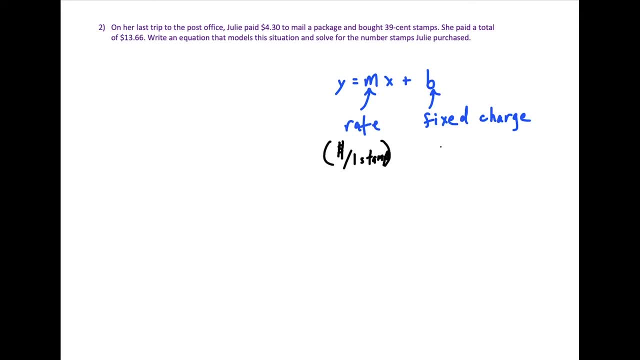 mail the package out. so that was a flat rate and this is the the cost to mail out the package. all right, that's not changing here. but just know, the amount she pays for the stamps depends on how many stamps she buys. that's why the rate attaches itself to the stamps and we're also told in this. 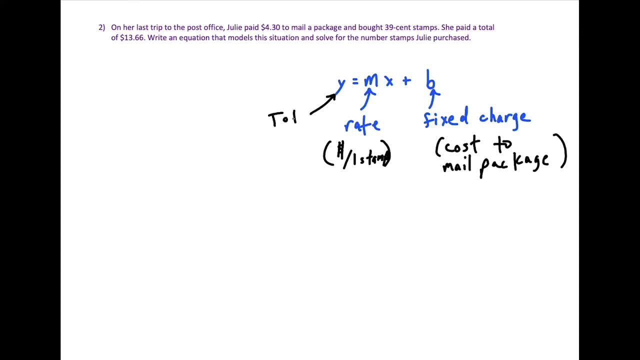 question here total amounts, so this is like the total cost of everything, and we know this information. so everything we've labeled so far was given to us and in this case, x is going to represent the number of stamps and that's what we're solving for. we want to know how many stamps. 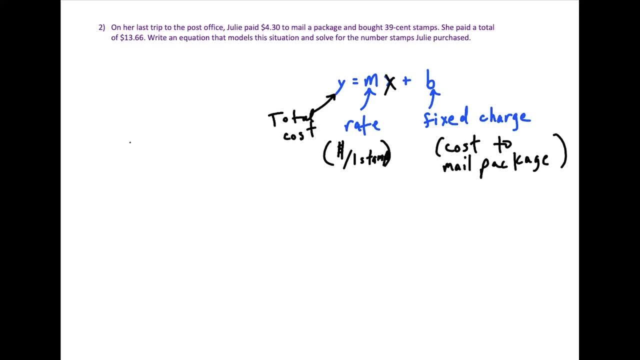 did julie in fact buy. so now we're just going to set everything up. the total cost of julie's trip to the post office was 1366.. so once again, we're going to write this without the units and then we'll interpret our answer at the end with the appropriate unit. so we have 1366 equals the rate. 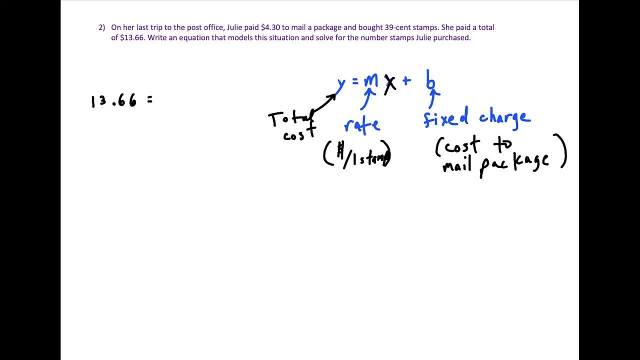 well, the stamps were 39 cents each, so the dollar amount per stamp is our slope or our m value. so that's going to go here. but just be careful, don't write 39, because 39 cents is .39. so once again, a tiny detail, but it can throw off the question. 39 cents is the same thing as .39. that's why we're 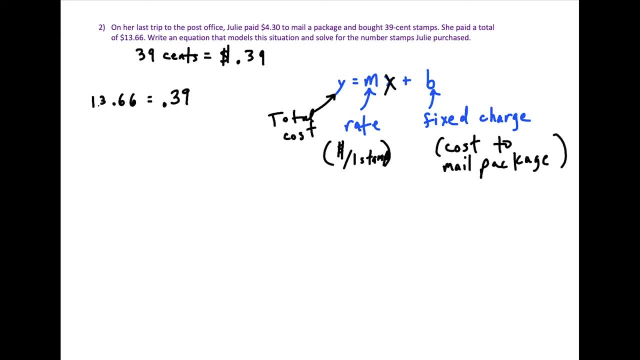 writing this as .39, so that the units match the thirteen dollars and sixty six cents. so we have point three nine times x, where x represents the number of stamps that she's buying plus the fixed charge. she paid four dollars and thirty cents to mail out the package. okay, so now all we have to do 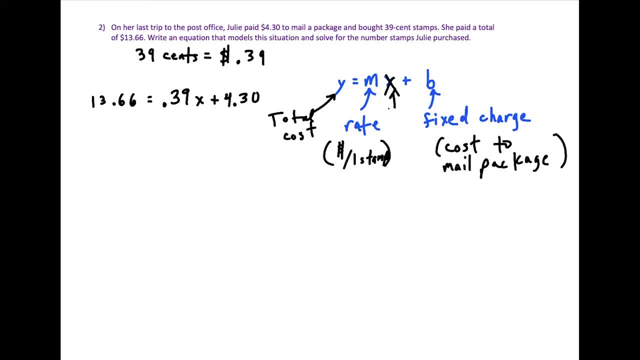 is solve for x, where x represents- once again this is the number, make that a little neater- the number of stamps. so the rest now we just solve this basic equation. we have minus 430 on both sides, and now we have 0.39 x. we could use a calculator here, but this subtraction isn't so bad, so we have. 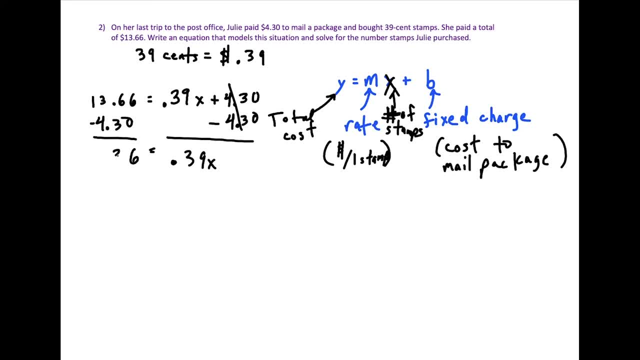 six, three and then thirteen minus four is nine. so we just bring down the decimal and then to solve for x, we're going to divide both sides by 0.39. so we could use a calculator here. um, i don't have one open just yet, so i'll just go ahead and do the division on the side. i'm going to write it as: